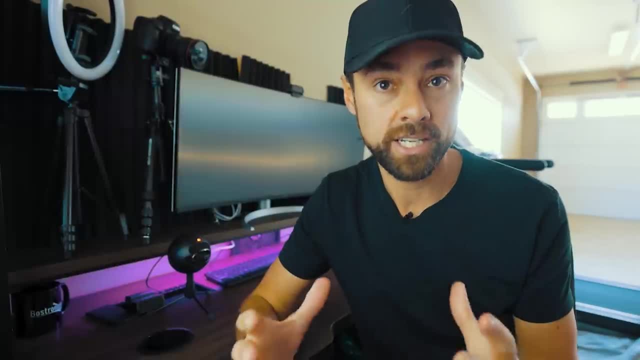 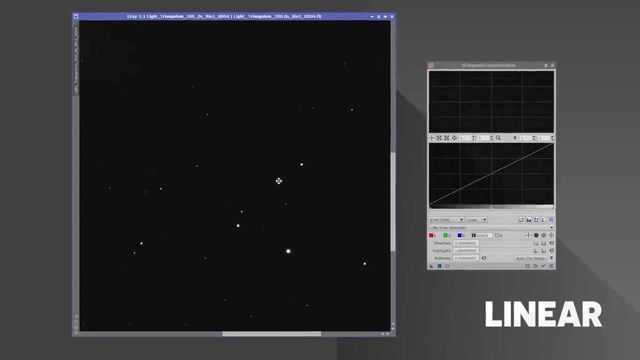 The first thing I want to explain is the idea of stretching an image. A single image frame that is straight out of the camera without any processing is known as a linear image. The histogram probably looks something like this, which just means that all the important data 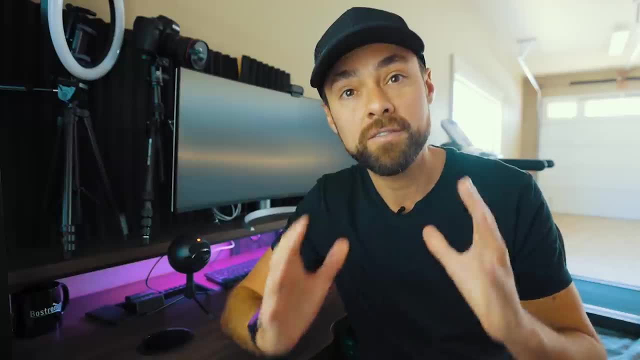 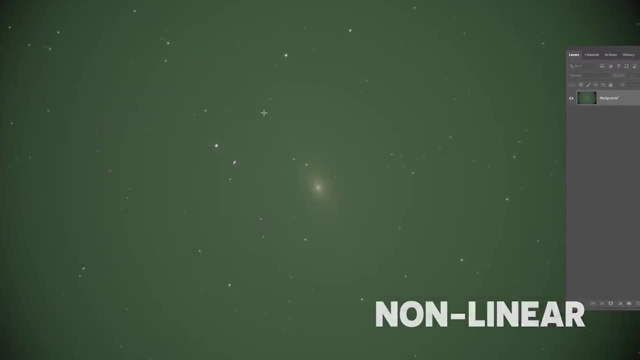 we want to reveal is crammed into this little wedge of information. A non-linear image is one that has had some sort of stretch applied to it or, for the Photoshop users out there, curves. Even a slight curve like this will brighten the image up significantly and you may realize that there's 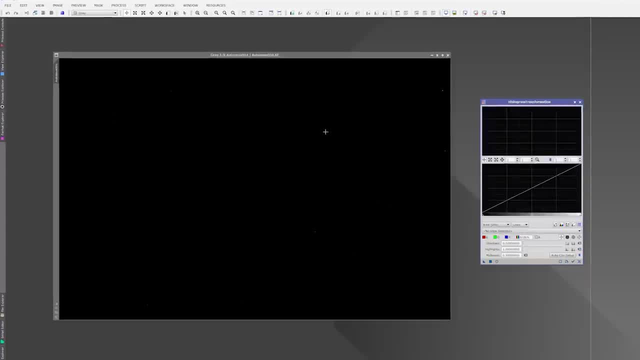 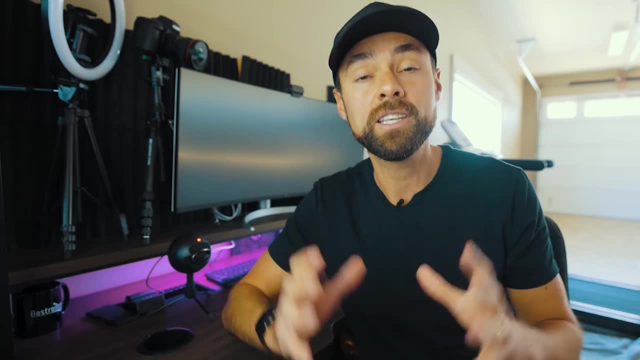 more information in that image than you originally thought. This black image you see here is completely normal. All of my images captured on a dedicated astronomy camera look this way when I'm starting out. Shots taken on a DSLR or mirrorless camera look a little bit better out of the gate. 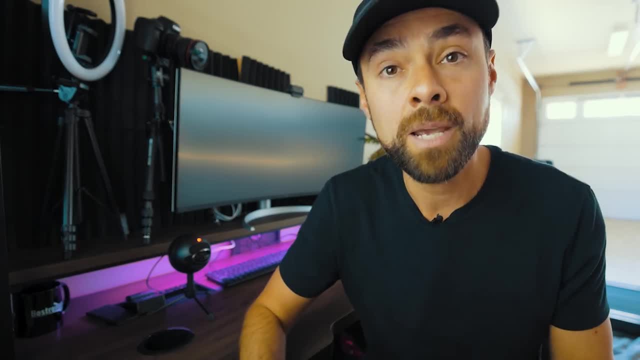 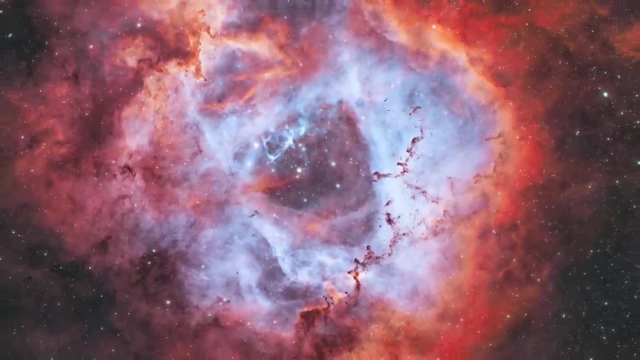 well, a little brighter. anyway, The point is, a single image frame is just a starting point for a much longer project. The final images I share in my videos include hours of exposure time and have gone through many hours of image processing as well. 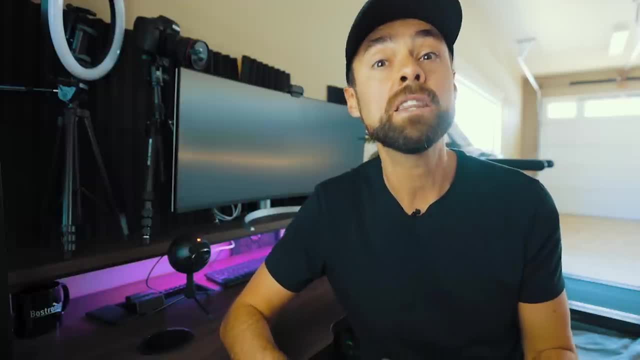 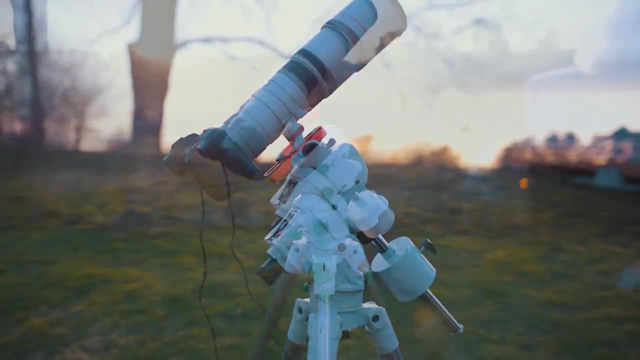 Let's talk about what you can expect your images to look like when taken through specific cameras and filters, because they're all different. There's a pretty drastic difference in the way a single exposure looks taken through a DSLR or mirrorless camera versus a dedicated. 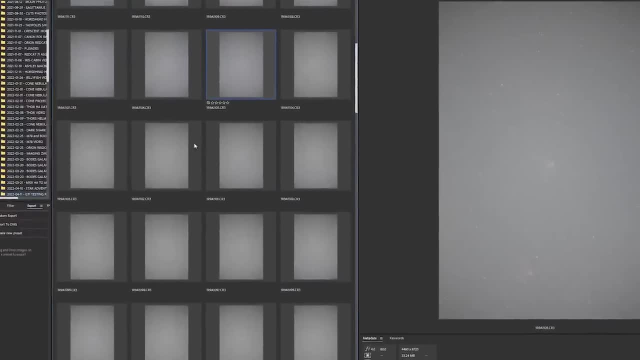 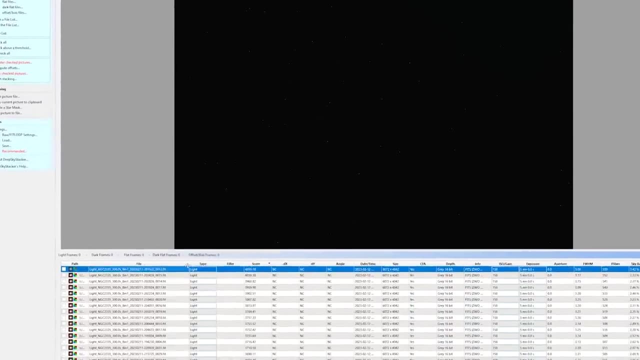 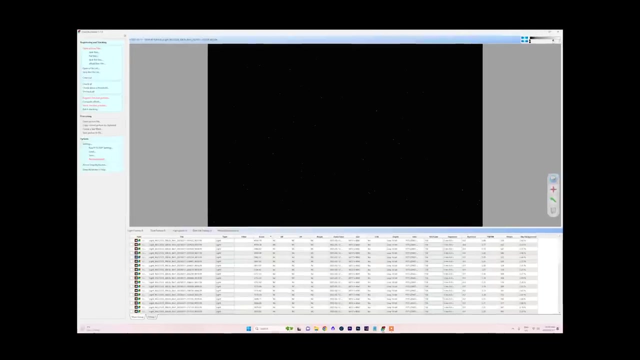 astronomy camera. The DSLR outputs a raw image format that can be exported into Lightroom or Photoshop for inspection, while the dedicated astronomy camera gives you these weird FIP file formats that you can't open up using a traditional photo editing software like Photoshop To see what you've captured using one of 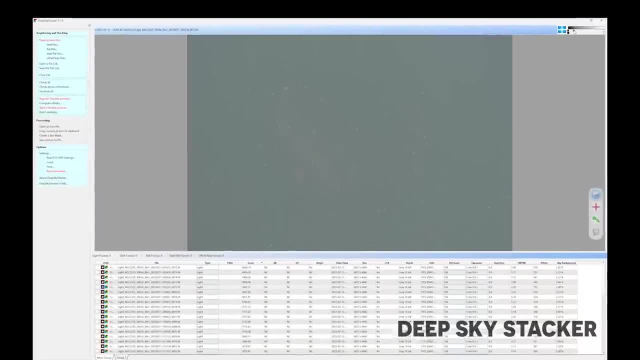 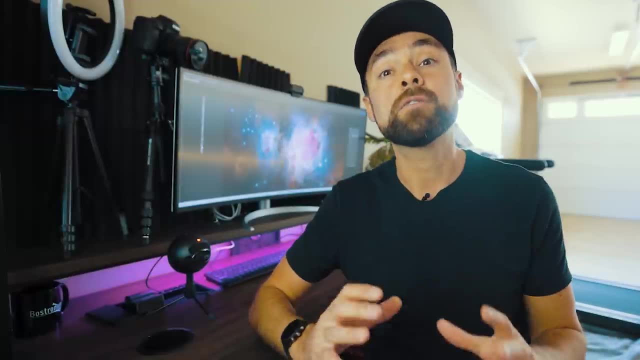 these cameras. you need to use an astronomy-specific software to open up the files and review them. I use Deep Sky Stacker, which just got a nice update, by the way, but there are many great free files out there that you can open up using these astronomy-specific file formats. 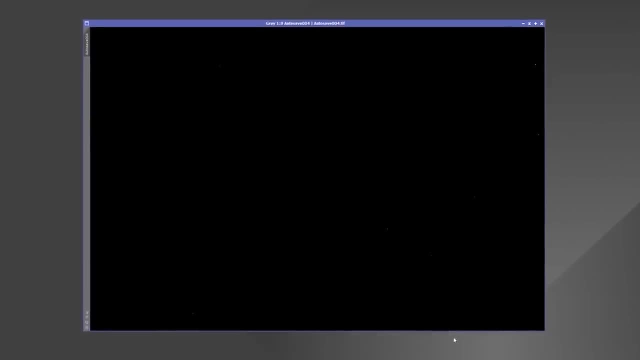 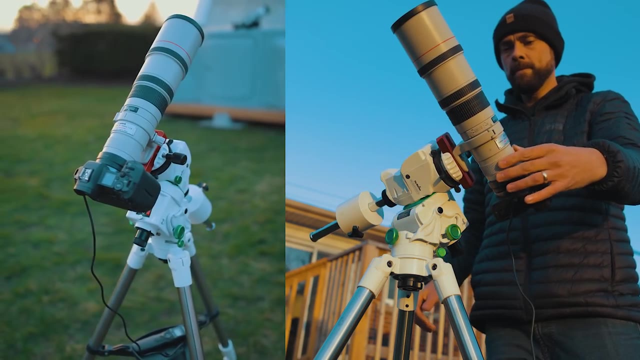 These images almost always look completely black in their linear state, depending on the camera settings and filters you used. DSLR and mirrorless cameras like my Canon EOS RA produce a brighter image in a raw format like CR3 that you can open up in a photo editing software. 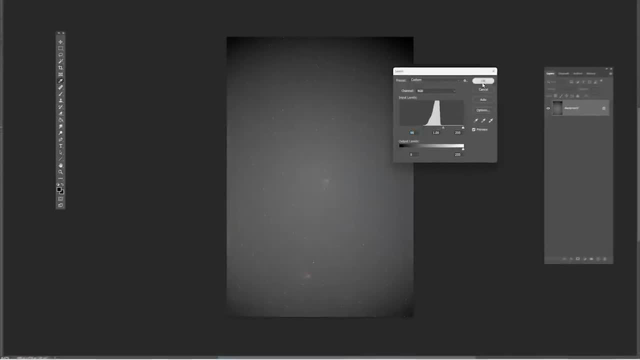 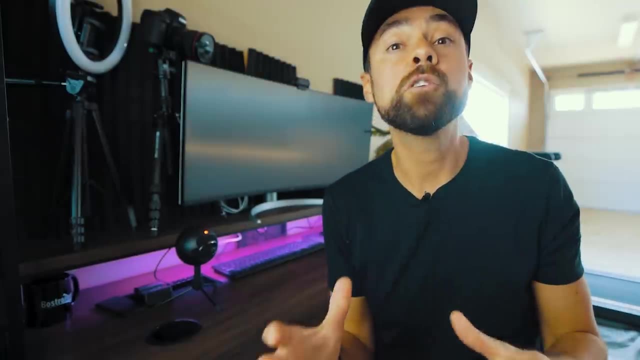 Although it seems like a much better starting point, more often than not, a single image frame captured with a dedicated astronomy camera will contain a cleaner, more detailed image. However, just like a FIP file, you can stack these raw image frames together to produce. 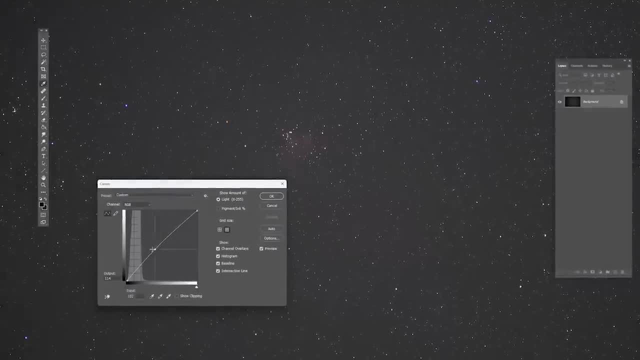 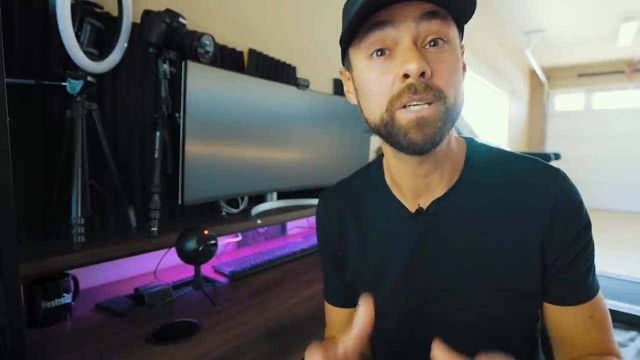 an image with a much stronger signal-to-noise ratio. The single frame might not look overly noisy now, but after three curved stretches the deep, dark, unexplored areas of the frame will be exposed. Astrophotography- image preprocessing- is all about creating that. 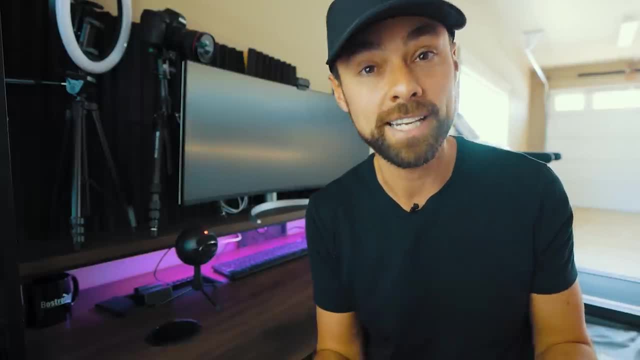 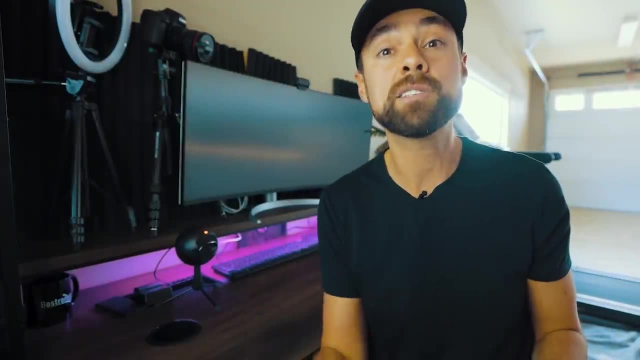 perfect master file that you can play with to your heart's delight without having to hide anything. Let's look at an example image in all three stages: A single exposure, a stacked master and the final processed image. The single exposure is boring, dull and dim. This is 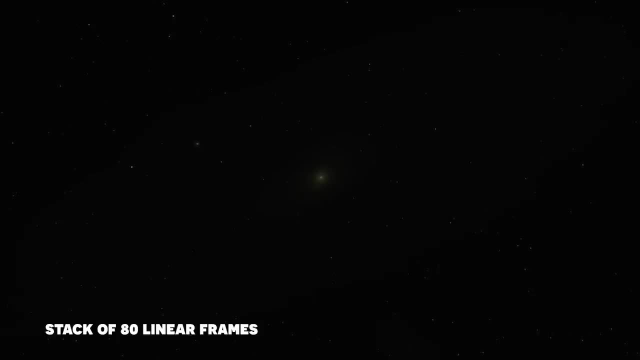 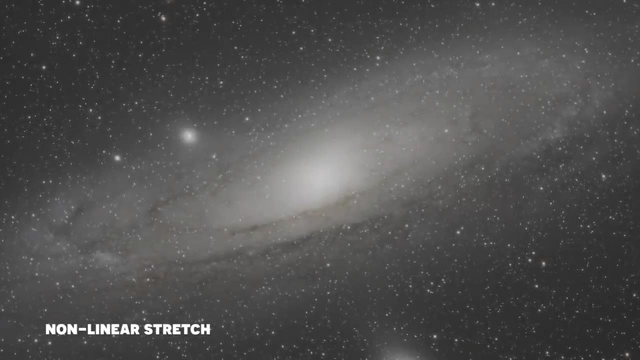 completely normal. The linear master isn't much more interesting, but you may actually see some faint cool structures going on now. Where it really gets interesting is when you give it that first curve stretch to bring up the mid-tones and highlights in the image. PixInsight has a really 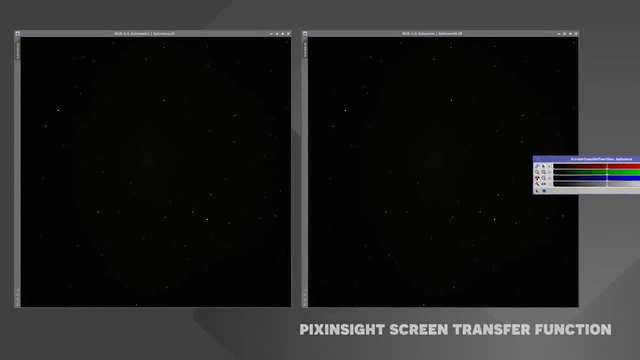 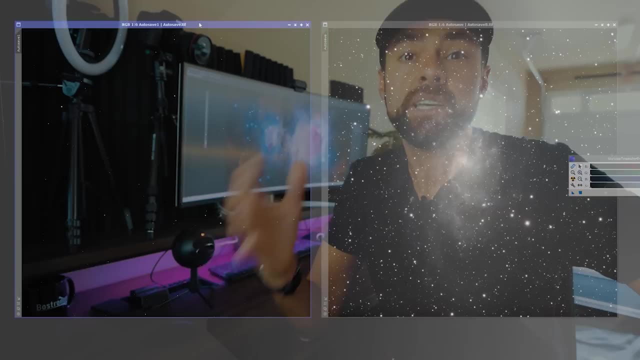 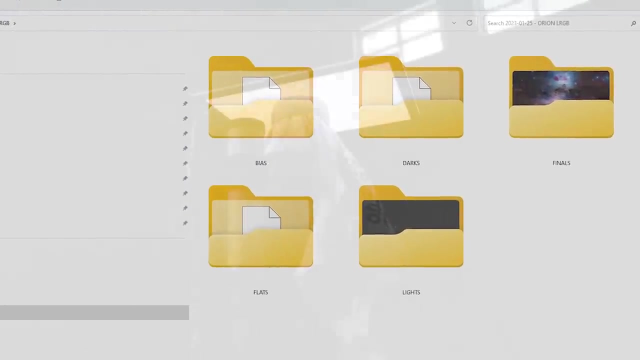 great tool to do this in an instant, and this is how cool it is. Just look at the difference between a linear and non-linear image. Pretty remarkable, isn't it? To get the best possible master file, there's a few extra things you need to do. Calibration frames are not the most fun thing. 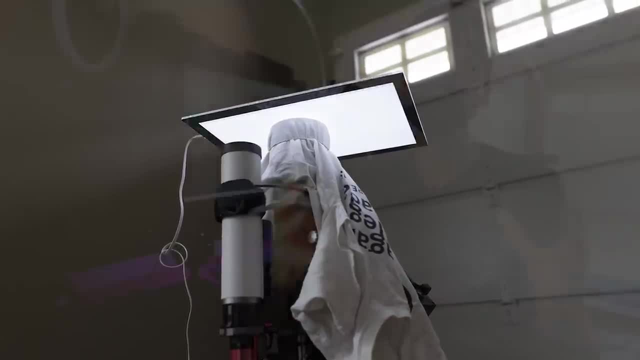 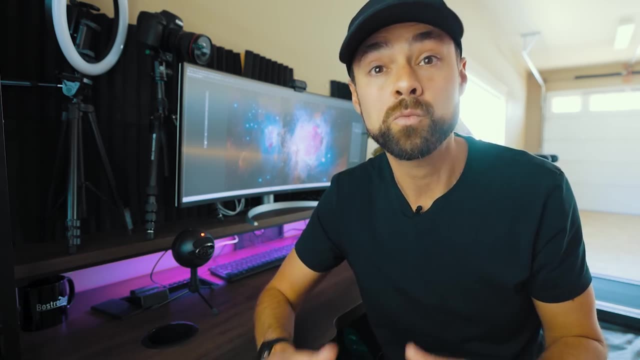 to capture, but they make a huge difference. I could make an entire video on calibration frames, but the bottom line is dark and bias frames help to reduce noise, and flat frames remove dust spots and vignetting. Do yourself a favor and capture these helpful files. It will make processing your 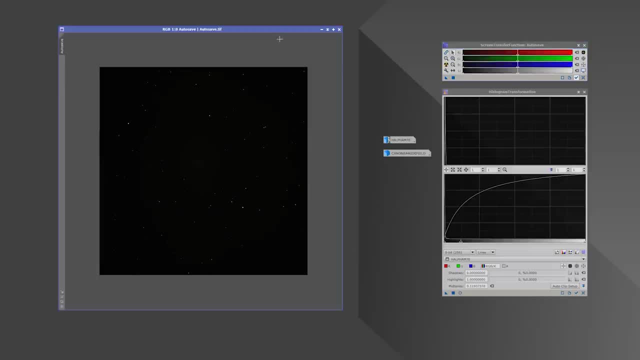 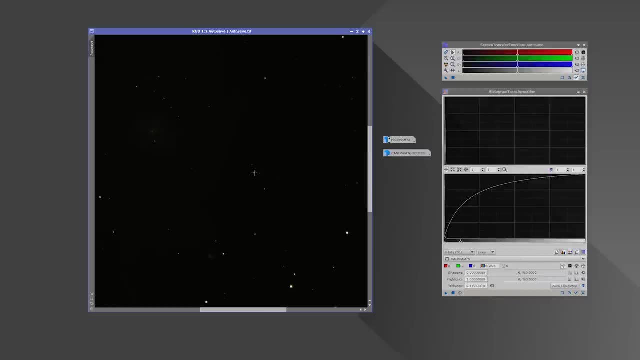 final master file a lot easier. If you're a master, you'll want to make sure that you have a lot more enjoyable. To recap, let's look at a few images taken with different cameras. The first one here is taken with a one-shot color dedicated astronomy camera, the 533MC Pro. 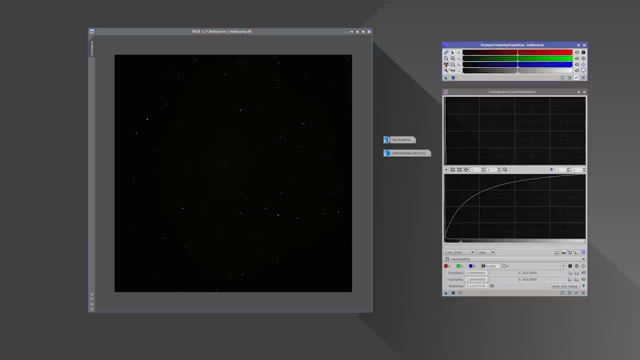 and again it looks totally black. this stack of images before we apply an auto stretch. So totally normal to see your stack and come out of DeepSky Stack or PixInsight- whatever you're using to stack- and to come out like this before any sort of stretching is applied. 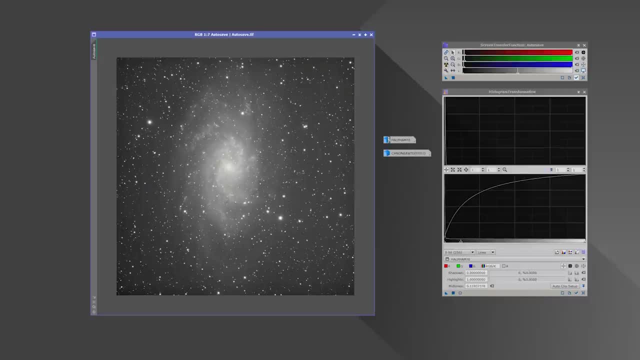 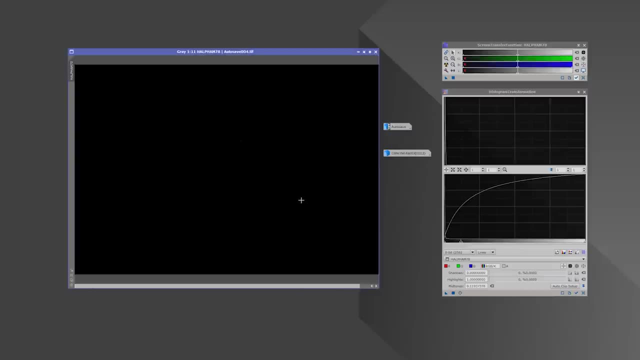 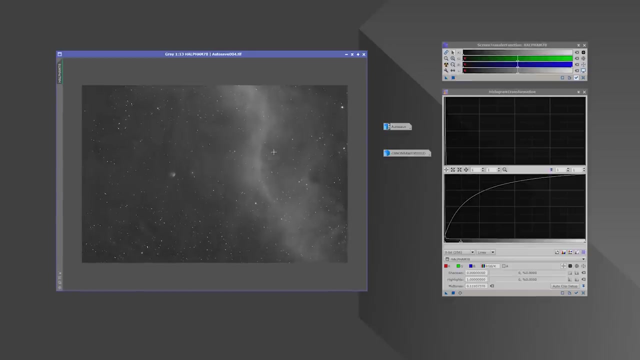 And it's linear state. If we look at a image captured with an H-alpha filter, there's even less going on in the linear state, just a black screen with a few dots. With the auto stretch to make it a nonlinear image, we can see there's so much information. 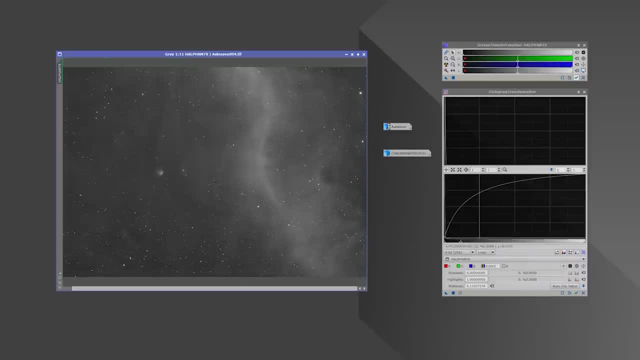 going on there and all of that info was crammed onto the left-hand side of the histogram, but it's just hiding in there, lurking in the shadows, waiting for you to find it. In our last video, we did a lot of work on the 10-inch screen, so I think you're going to enjoy this video. If you've enjoyed this video, please let us know in the comments down below. It's a really, really helpful and helpful. We hope you enjoy it and we'll see you soon. Bye for now and I'll see you next time. Bye. 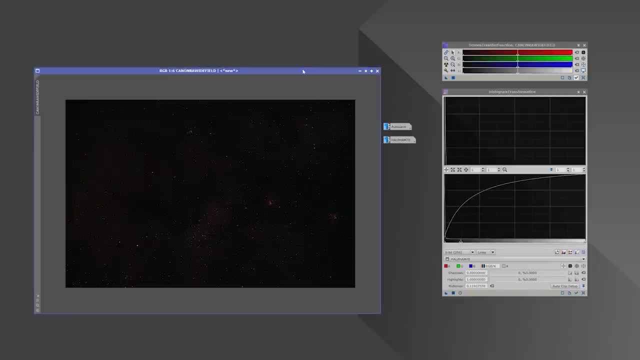 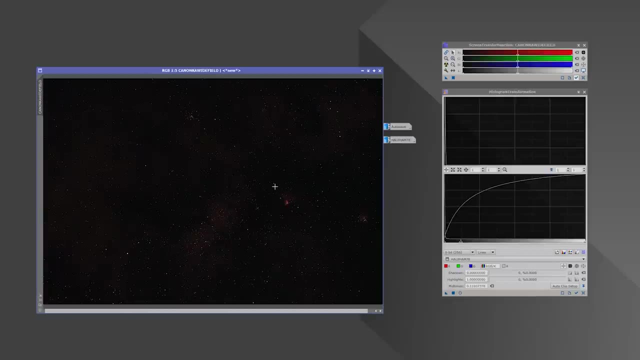 example- this was taken with my Canon EOS RA of a star field in the Milky Way, and with a camera like this you can see a little more. in the single image frames and the stack you can see a few deep sky objects, but it's still very dark If we 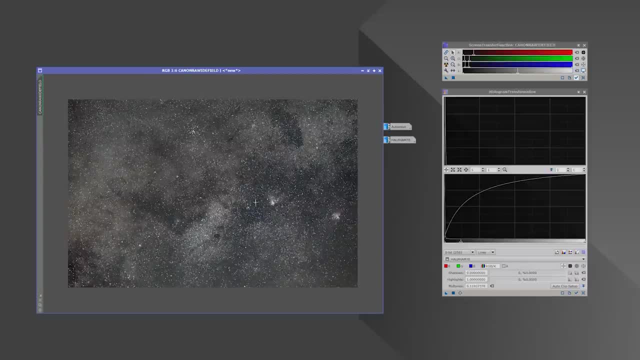 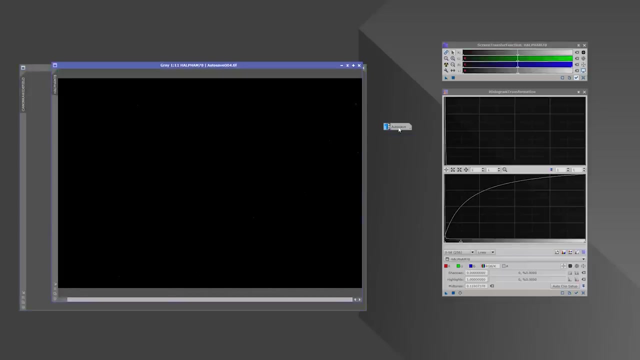 apply a quick auto stretch to this, you'll see there's so much more going on, and all that information was just lurking in the shadows of the histogram, waiting for you to pull them out. So, again, get used to seeing images in this really dark state once you stack them and know that there's nothing wrong with. 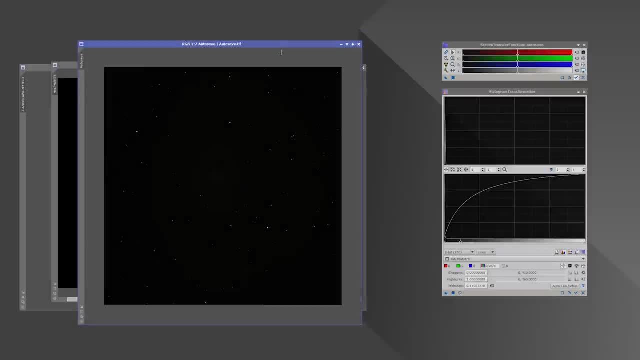 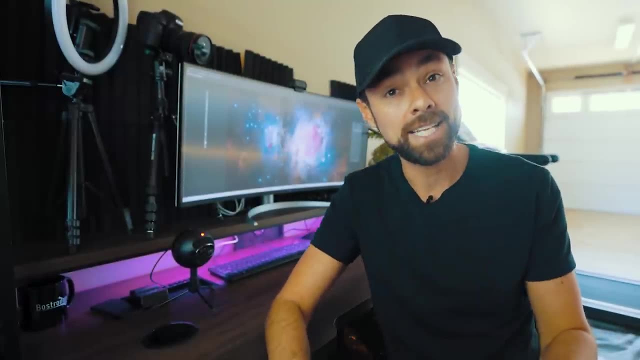 your camera. it's just a matter of a linear image versus a nonlinear one. I hope this video has given you a better idea of what your images should look like after you take them and, more importantly, put your mind at ease when you see that first image. that's all black with a couple of white dots, with 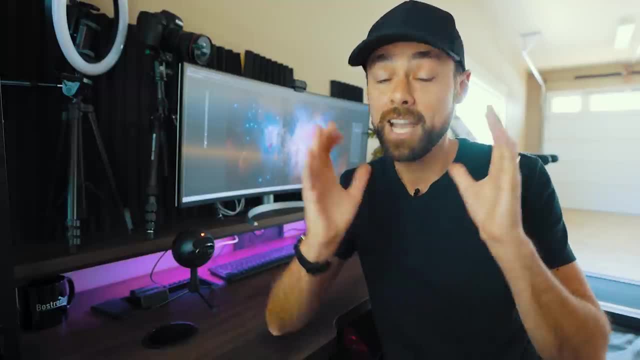